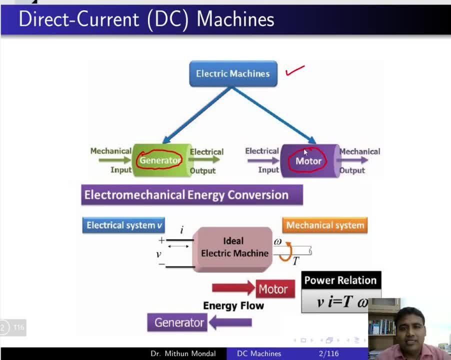 So when we talk about generator or motor in DC, then it is known as electrical machine, or in AC as well. So when the mechanical input is given and the electrical output is taken, then it is known as a generator. When the electrical input is given and the mechanical 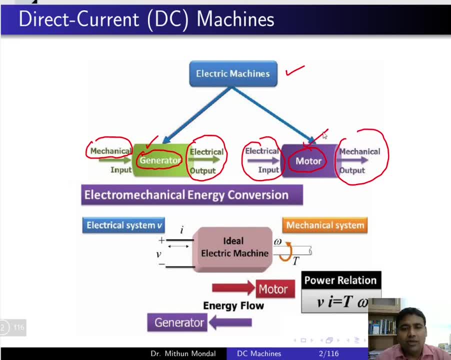 output is taken, then it is known as a motor. Both generator and motor can be tell to be as a DC machine. Now, these are electromechanical energy conversion devices, Because electrical energy is converted to mechanical energy, or mechanical energy is converted to electrical energy In the ideal electrical machine. ideal means there is no. 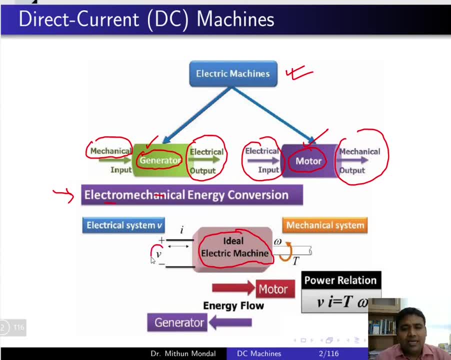 losses. So if you are giving an electrical energy in the form of a voltage, you are able to rotate the shaft of the machine, So a mechanical power is generated. On the other hand, if you reverse it right, If the reverse the energy flow, then it will operate as a generator. 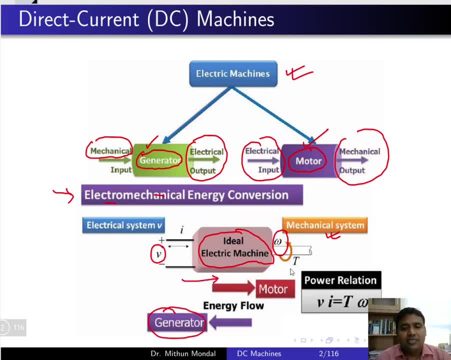 So in this way, when electrical energy is given to rotate the shaft of the machine, then it is operating as a motor. when you are giving the mechanical energy to get the electrical output, it is working as a generator. So the power relationship, So the power relationship will be voltage into current is. 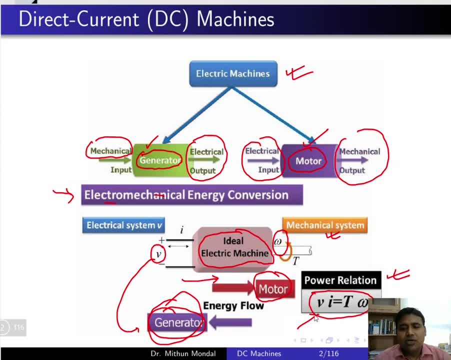 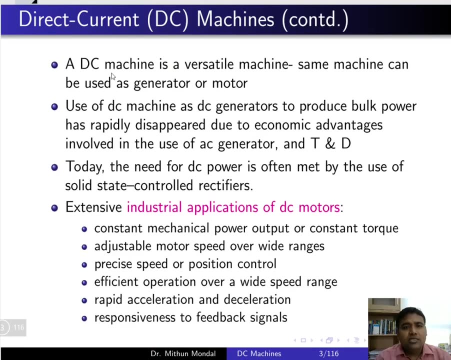 is equal to torque into omega. So voltage into current, that is the electrical power, and torque into omega is your mechanical power. So under steady state condition your electrical power will be equal to your mechanical power. Now, DC machine is a versatile machine, So why? 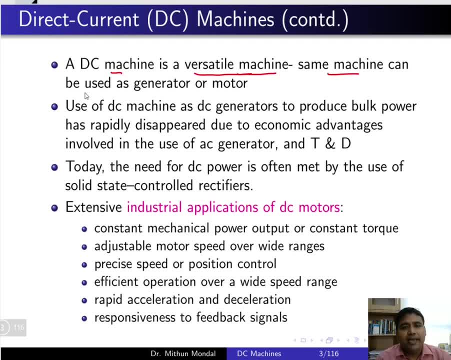 I say it to be a versatile because the same machine can be used both as a generator as well as motor. So when we use DC machine, the same machine can be operated as a generator or a motor, depending upon the energy flow. So use of DC machine as DC generator to produce bulk amount. 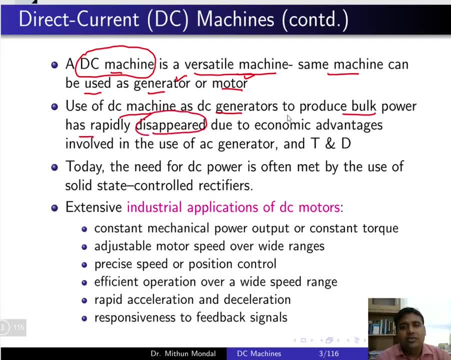 of power has rapidly disappeared due to the economic advantages involved in the use of AC generator and transmission and distribution. So this point I was also discussing in the electromechanical energy conversion device, that when DC machine nowadays it is not operating as a generator because the we require to produce. 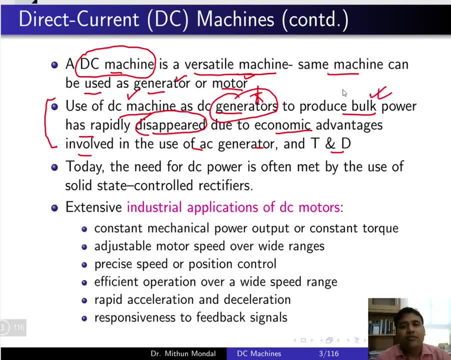 bulk amount of power, which is not possible with the help of a DC generator because the cost will increase a lot. So in this case, for the economic advantage, we will be generating energy with the help of an AC generator and then, if DC power is required, then we will convert the. 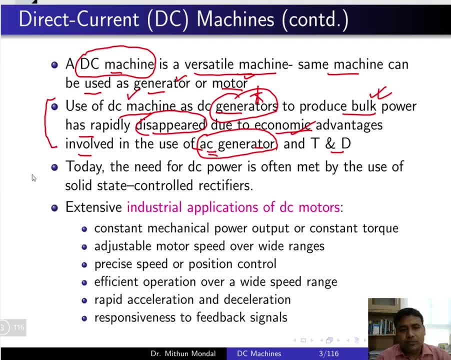 AC power into DC power. So today the need for DC power is often met by the use of solid state controlled rectifiers. So this also I have discussed that in order to produce the electrical energy we produce in the form of AC. that is what AC generators are used nowadays. DC generators have 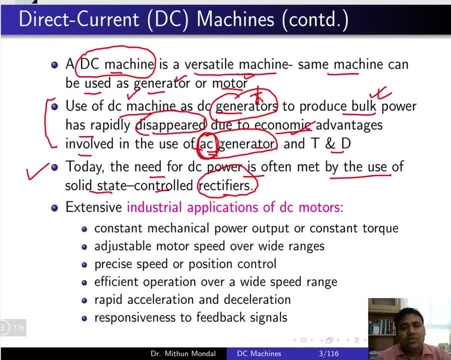 become obsolete. Now, when the power is generated in the form of AC, then it will be used as a DC generator, and then it will be used as a DC generator. So this is a DC generator and, using the solid state controlled rectifier, we will be converting the AC power into. 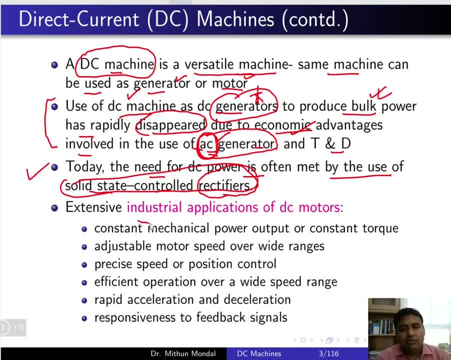 the DC power. Next, some of the industrial application of DC motors. Let us see the industrial application of DC motor. So first application is constant mechanical power output or constant torque. So such type of places where you required constant output power or you required constant torque, then this is one of the important application of the DC motor. Now please look at: 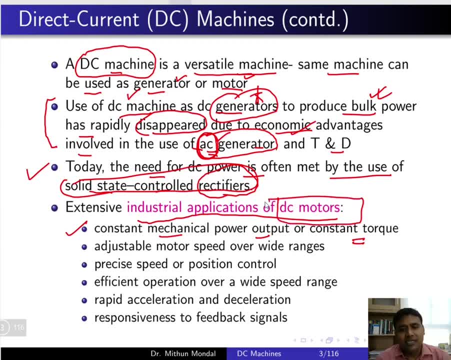 this. look, we are focusing on DC motor rather than DC generator because, as I said, whenever I will be talking DC machine, nowadays it has become analogy to DC motor, only not the DC generator. Second application is adjustable motor speed over wide range, So you can control the speed over a wide 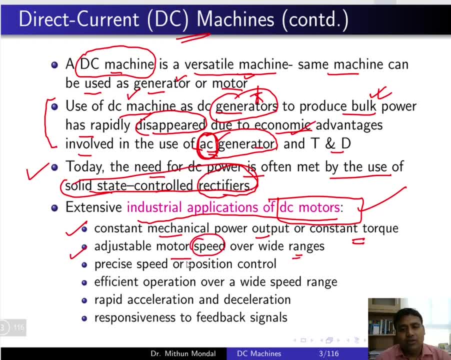 range. So whenever you required to change the speed of the motor, you can do it. Then precise speed or position control. So whenever you require to change the speed of the motor, you can do it. Whenever you want to like control and see, stop or start the motor, then you can do it efficiently. 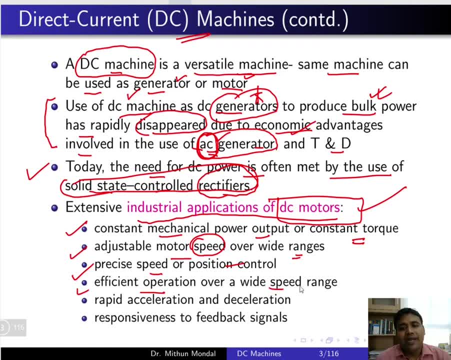 Next, we have efficient operation over a wide speed range. So this motor efficiency is quite good. over a wide speed range, Rapid acceleration and de-acceleration is possible. and responsiveness to the feedback signal. What is the meaning of feedback signal? Now, if you see, if there is a? 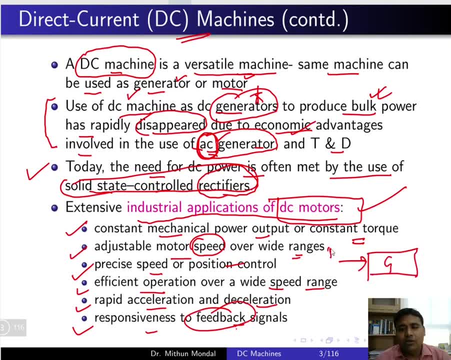 plant G, then if you are giving an input and taking the output, so this is without a feedback. However, if you connect one more system here H and connect it with here, then it is known as the feedback, So whatever the error signal you are getting. so here we have connect the error signal, So same error signal will be given as 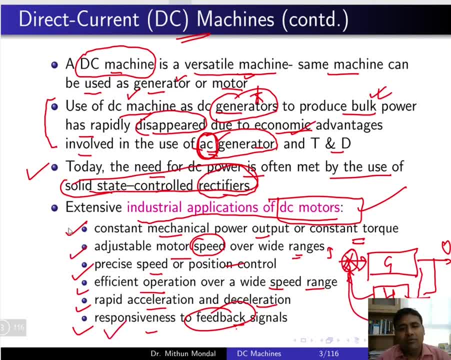 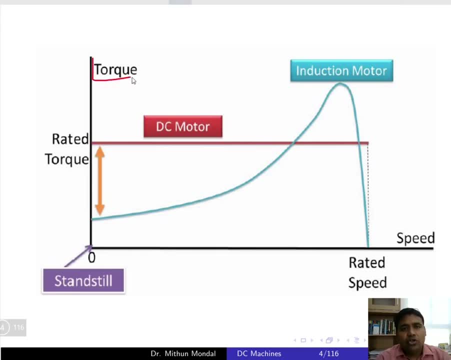 the feedback, So it has a good responsiveness to the feedback signal. So these are the extensive industrial application of DC motors, because it has a lot of advantages. Now, if we draw a curve between torque on the y-axis and speed on the x-axis and then compare the DC motor with one of the most famous AC motor, that is, the induction motor, 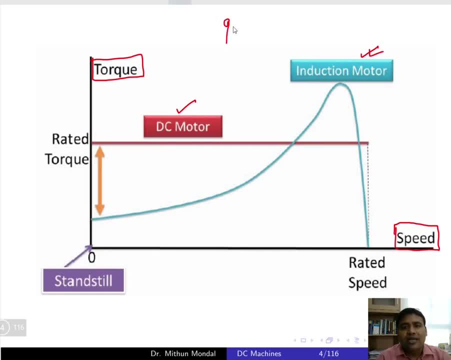 Now, at this point of time, I would like to say you that around 96 to 98 percent of the motors that are used in industries are basically the induction motor. Okay so, in industries, if you see, the induction motors are the one which is mostly used. Induction motors are basically the AC motors. 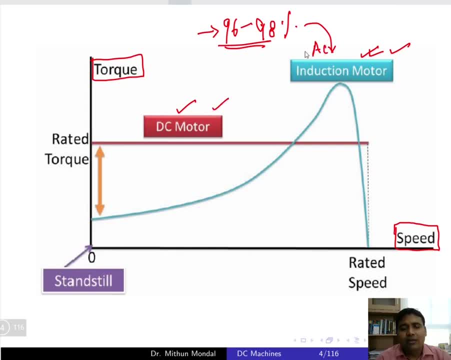 So let us compare the DC motor with the, with AC motors in terms of its characteristic torque and speed. So here it indicates the standstill operation. The motor is stopped at this position, standstill. Then what we see? that at the standstill position, if you start the motor, then the rated torque, that just the beginning of the start, if you compare. 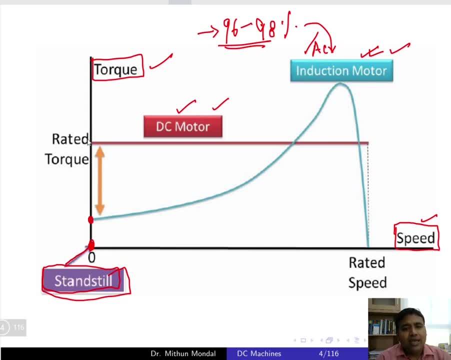 the rated torque of an induction motor with the help of with that of the DC motor, then we see that the rated torque of DC motor is quite high then as compared to the induction motor. So at the beginning the rated torque of the DC motor is quite high as compared to induction motor. 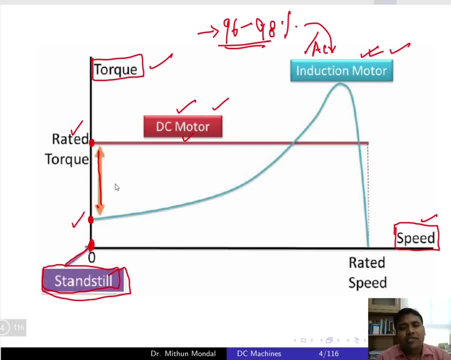 So in such type of application, where we required to start the motor with heavy load, then we should not use induction motor, rather we should go with DC motor, because its starting torque is quite high. Now, as the motor gathers speed, we see that the torque of the DC motor is quite high. 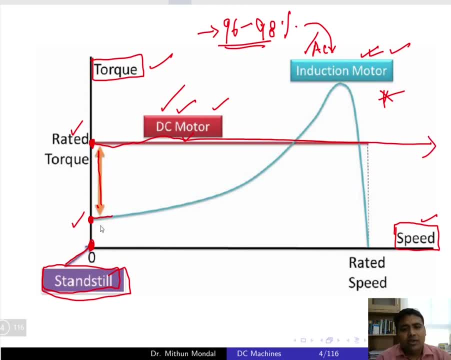 motor is constant, whereas the induction motor slowly gathers the red torque and then it reaches the maximum position and then it drops. Now why 96 to 98 percent of the industries using induction motor? there is the reason, because is that two important advantage? I will be just 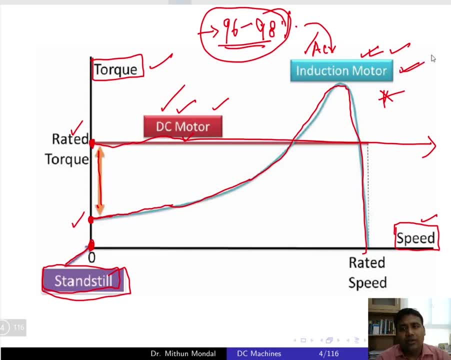 pointing out at this point of time for induction motor. induction motor are self-starting motor. self-starting means we do not require anything extra item to start the motor. that is, we are talking about three-phase induction motor because AC motor can be single phase or three-phase. so 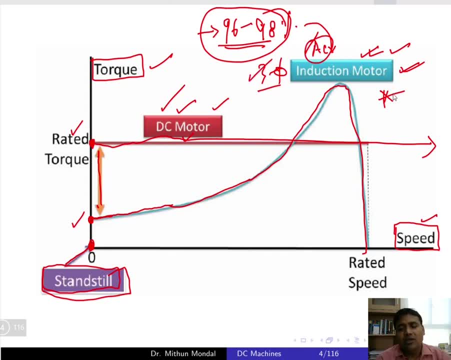 most of the industries are using three-phase induction motor and three-phase induction motor are self-starting. Moreover, three-phase induction motor is very versatile in nature. it can be used in robust. it can be used in any like industries. apply applications like where you will be seeing. 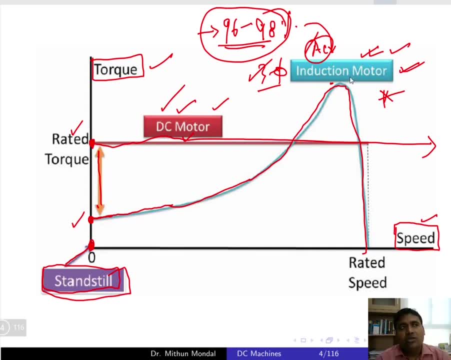 in cement industry there will be a lot of pollution, or some gun industry where there is a lot of- you know- severe happening there. so in such type of application induction motor is the one which is mostly useful. so because of the advantage of induction motors we generally use induction. 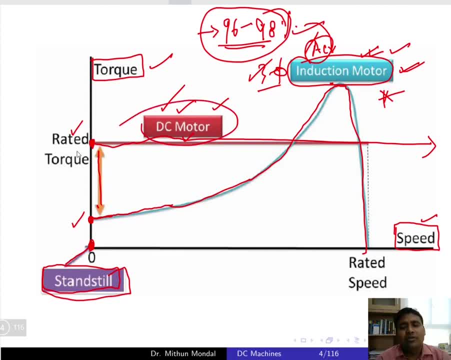 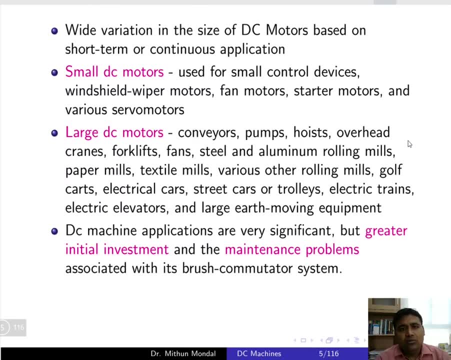 motor in the industries. How is it used? How is it used, However, DC motor have got their own advantage because the rated torque is quite high for the DC motor. Now let us see the classification of the DC motor. so the wide variation is that of the. 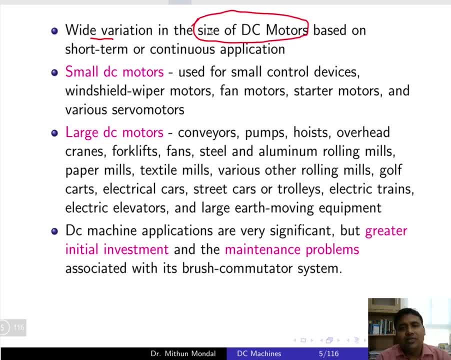 size of the DC motor. so if you see the size of the DC motor, there is a wide variation and that is based on short time or continuous application. okay, so you will be having small DC motor, large DC motor or it can be very, very big motor, So small DC motor. so when we are talking about the 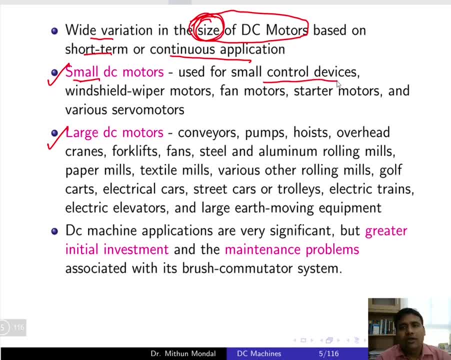 size. small DC motors will be used in small control devices, wind shield, wiper motors, fan motors, starter motors and various servo motors. so these are small DC motors where, as the large motors, if you see, then it will be use in conveyors, pumps, worst overhead cranes, forklift fans, steel, aluminium rollings. 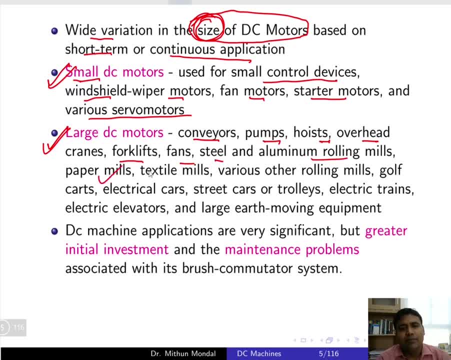 and lot of other appliances, like you can see, which is written: paper mills, text triangles and various other things. so you can see that if you talk about an elevator or you are talking about a waste pump or you can talk about some electric cars, so you can see the weight will be very high. so if the weight is, 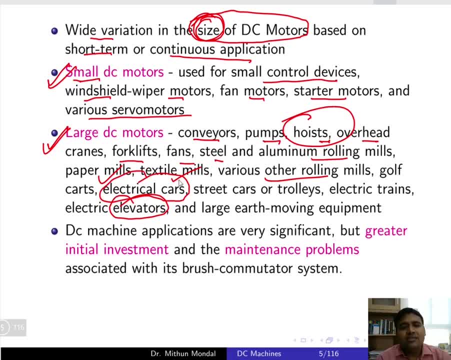 very heavy, then in that case the starting torque requirement should be very high. so in such type of applications we prefer to use DC motors rather than the induction motors. so in these type of applications you can see that the starting torque will be very high. it will be requiring due to its 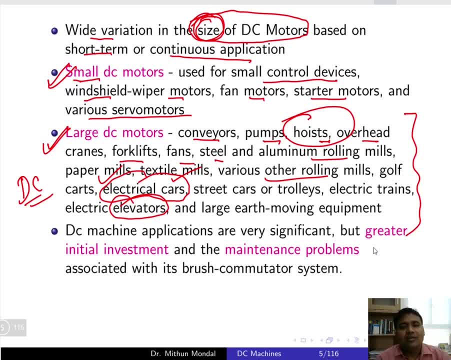 loading. we will be using DC motors rather than the induction motor. next, proper point: DC machine applications are very significant, but greater initial investment. now this is one of the important limitation in DC machine. your investment, that is initial investment, will be quite high and there will be maintenance problem because we 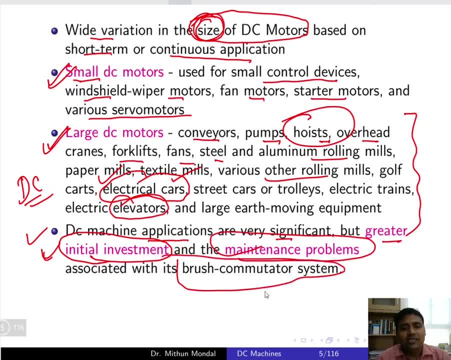 will be using a brush: commutator segment. now, what is a commutator? what is a brush that we will see in the construction? so, at this point of time, you just remember that the initial investment of DC motors or DC machines is quite high and it 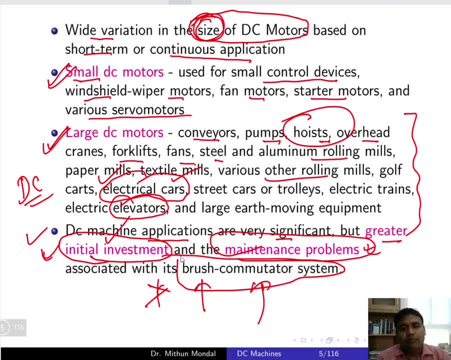 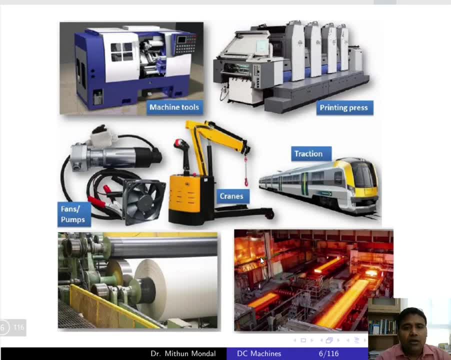 require frequent maintenance issues because of brush commutator segment. now, what is a brush or is a commutator? that we will discuss now. if you see the application of the DC motors or DC machines, so DC machine and DC motor analogic will be using every. 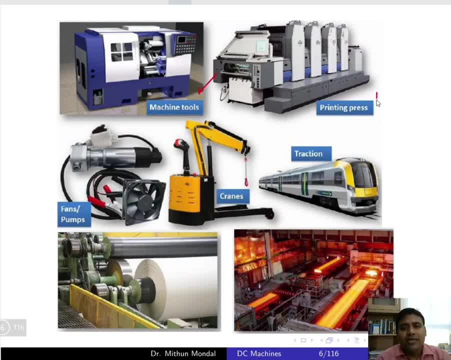 time. so you can see in machine tools, printing press, traction cranes, fans and pumps, rolling wheels and paper mills. in these type of applications we use DC motors. so everywhere you will be seeing see that heavy load are associated. so when heavy load is associated, then the rated torque 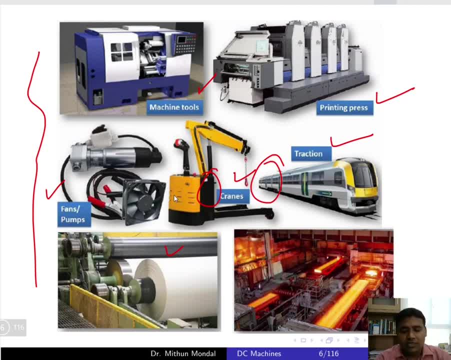 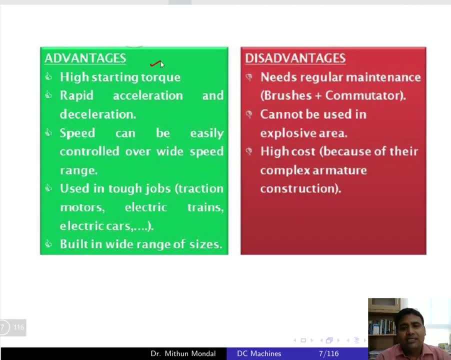 has to be high at the beginning, so DC motors are preferable. now let us compare the advantages and limitations, or disadvantages, of DC motors. so DC motors had high starting torque. remember DC motors will have high starting torque, which is the main advantage of the DC motors. second, it: 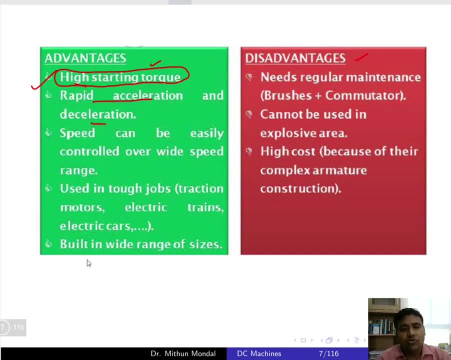 will have a rapid acceleration and de-acceleration. so you have seen the curve of induction motor. so if you draw the curve of induction motor torque speed, then with the speed the torque is gradually increasing slowly and then reaching the maximum position. however, the DC motors are constant. so rapid acceleration and de-accelerations. 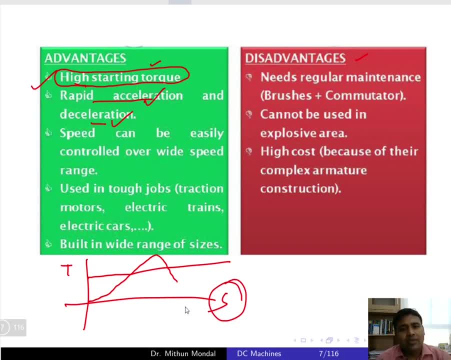 are there because it can gather a speed quite high and reduce also. so this is the second advantage. third advantage: speed can be easily controlled over a wide speed range. so when DC motors rotor rotate, then you have to control this speed and there are certain methods to control the speed, which we will be. 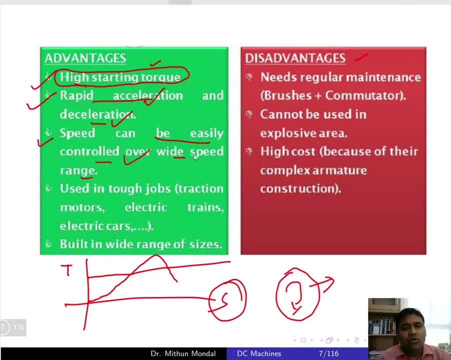 learning. it can be easily controlled over a wide speed range. fourth one: use in tough jobs- traction motor, electric trains, electric cars- so these are very tough job where high starting torque is required. so they are used and built in wide range of sizes. so if you see a DC motor, it can be very small size and it can be very big size. 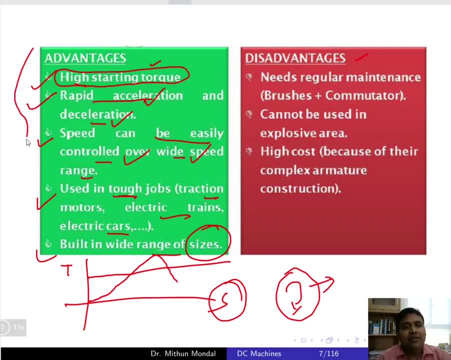 even used in the industries. so these are the advantages of the DC motor. now let us point out the disadvantages or the limitations. now, the major problem that DC motors have is due to the presence of brush and commutator. so due to the presence of brush and commutator, it is requiring regular maintenance. so we would 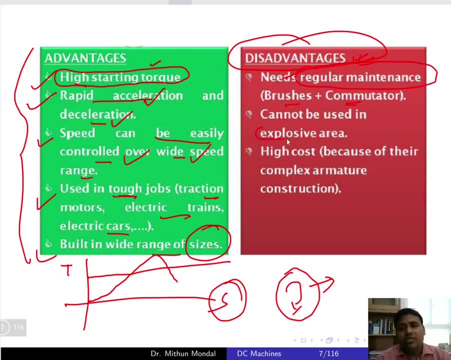 be requiring regular maintenance and it cannot be used in explosive area. so that is what I was talking in induction motors. they are more robust and hence it can be used in any environment where, as the dc motors cannot be used, so explosive area dc motors will be not used and the costing is. 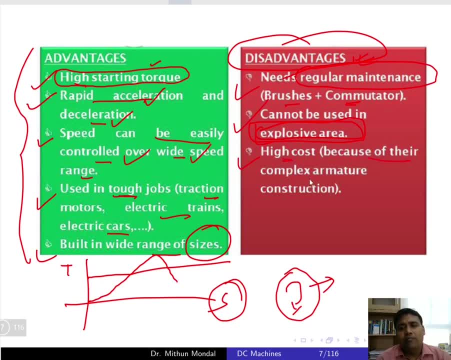 again an issue. it has high cost because of their complex armature construction. so, armature, what is an armature? what is a commutator? that all things we will look at this point of time. you just remember that the cost of the dc motor is high because the armature construction is quite high. 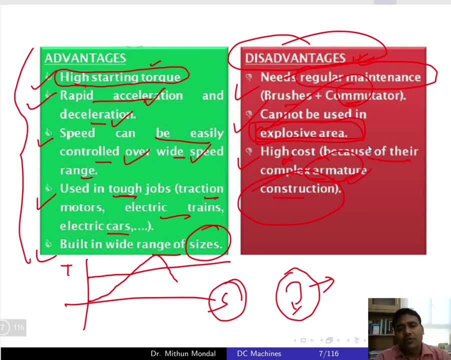 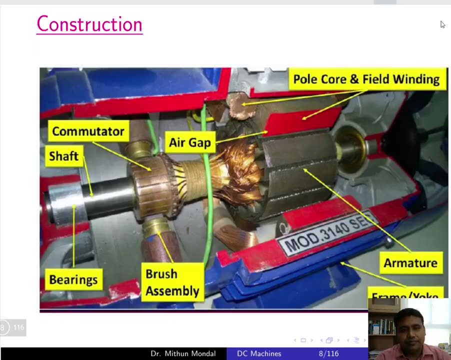 so armature is basically the winding which is present in the dc machine. so advantage and disadvantage of the dc machines is very important, of the dc motor is very important and because, based on that, we will be using the dc motors in different applications. now let us quickly look. 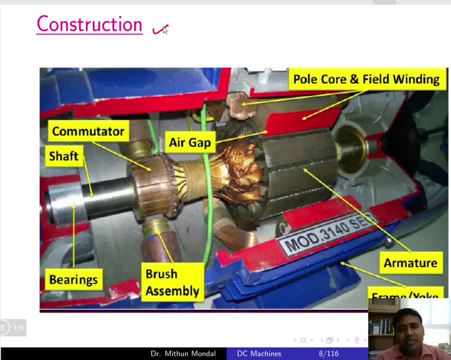 into the construction of the dc motors, which we will again discuss in detail. so at this point of time i will show you the construction of the dc motors, which we will again discuss in detail. would like to say that the dc motor will be having two important parts. one is known as the stator. 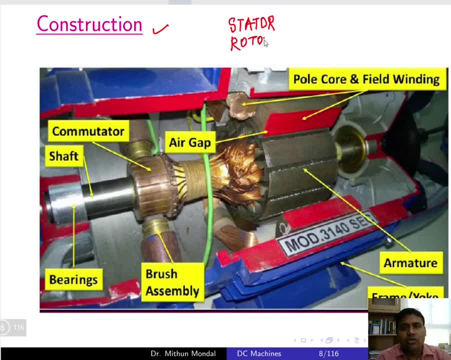 and other is the rotor. so there are two important parts of a dc machine. one is stator and other is a rotor. so stator, as the name suggests, this is stationary. so something which is stationary is a stator and something which is rotating or moving is a rotor. so dc motors has two important part: one is stator and other is a rotor. 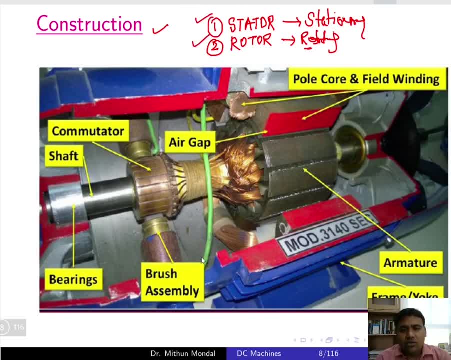 okay, so let us quickly look the important parts of a dc machine, what we have. so here you can see that there are the windings that are present. so you know we have discussed that any production of torque can be possible if we have a dc motor which is moving, or moving is a rotor. so dc motors has two. 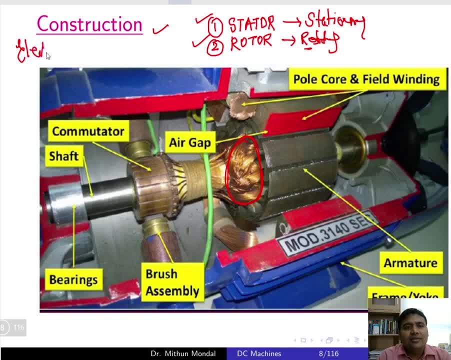 important parts of a dc: the stator and any other instrument, and that is a rotor, which is a rotor, along with there is a rotor type cylinder shaft which is approximately only 300 Arabic thousand, one Style wheel bar. if there are a steel двигator, this is generated by the electric currentAngles, magnetic field and magnetic field. so both will require current as well as magnetic field to produce the torque. current, magnetic field interaction is very important to have the production of the torque. now here, this is an armature, so this is the armature. so the winding during the electric current, electric leak, will Jak the electric cancer. is very important to have the quality of the electric filter in finishing the electric speed while at the same time it 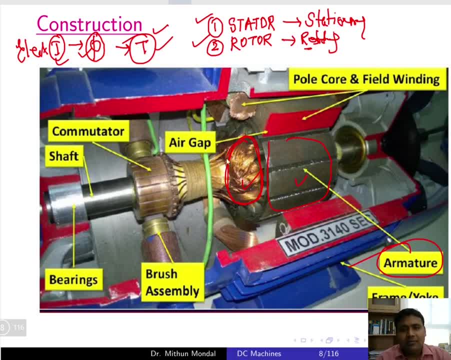 is present in the armature in some connection. what are the connection that we will do? and the field is produced with the help of the poles. so this is basically the poles that is present. so this side and this side- both are poles- are present. so we have seen this is a north pole. 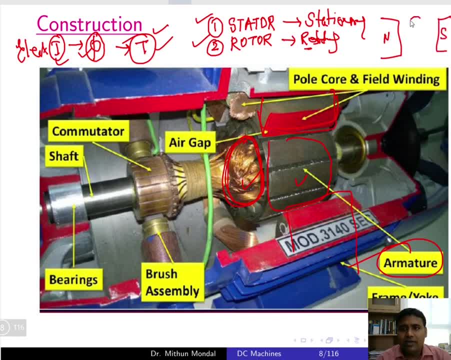 and this is a south pole, and you have an electromagnet which is rotating right. so Faraday's law states that emf will be produced only when there is a relative motion right between the flux and the conductor. now this relative motion can be produced by either: 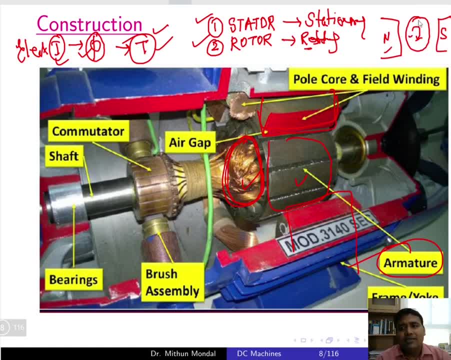 rotating the magnet, moving the magnet, keeping the conductor stationary, or rotating the conductor, keeping the field stationary, any of that. so in dc machine we will be keeping the field constant. now, remember, in dc machine we will be keeping the field constant. so in dc machine we will be. 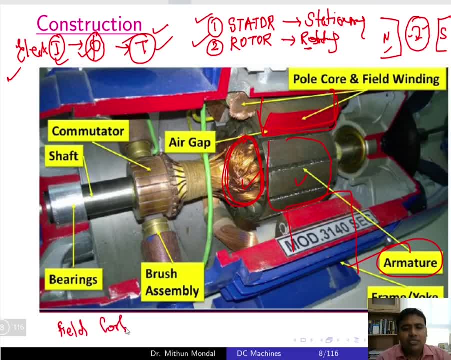 we will keep the field constant or stationary and we will rotate the conductor. so the conductor will be rotating. okay, just remember, because this is accordance with Faraday's law, because we have to produce the emf or the torque. so either we tell emf or torque for a dc. 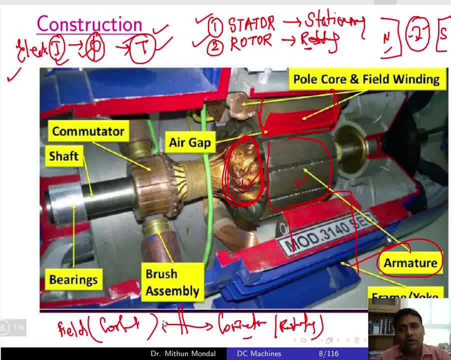 machine. it is basically means whether it is a generating end or the motoring end, motoring mode, the interaction of current and flux has to be there to produce the torque and there should be a relative motion. so relative motion can be produced by either changing the field moving, 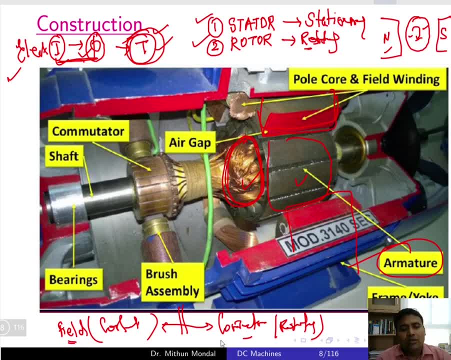 the field, keeping the conductor constant, or moving the conductor, keeping the field constant, anything. so in case of a dc machine, remember, the field will be constant. field will not move or not rotate anything only rotating part will be the emf or torque. so this is a class which is we can choose not to constantly change the price. what we are doing here is 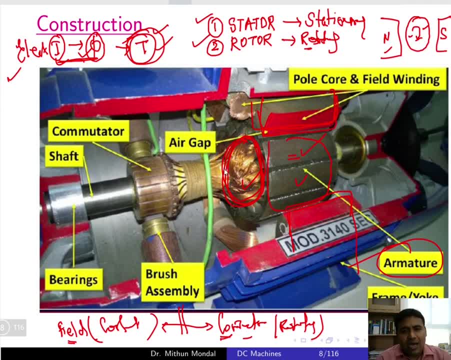 that the forecast. that is good now if you think. touching the aha when you do a show is good now. let us now think about the涵, multiple pros and cons of the Dc phase section. what is the partnership between two business and formula signal, one of its manytered and 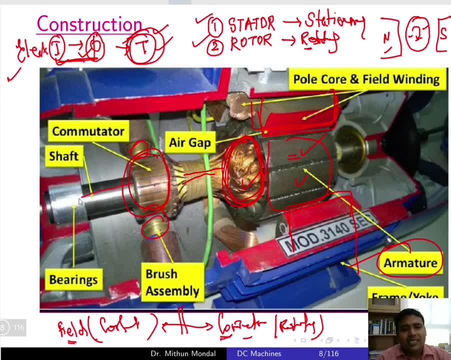 two Laplace 없어요 when simply mentioned that the based on an emf product share would be correction of the energy flow through to the Dc to Dc and we issue the families of the B air supply and so our environment. so the compañía central musical Kyle that we 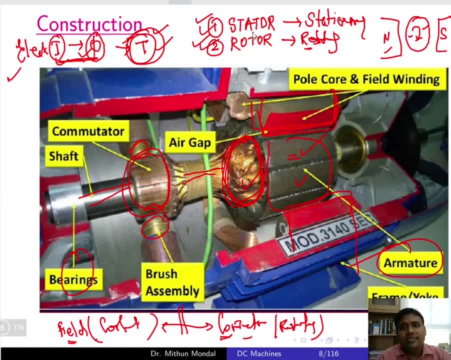 receive right when we a function we provide in the management. also, we are not commercially doing so- all this may not be a у and so, for example, for a household with purchased dust. So first you remember stator and rotor. stator is the stationary part, rotor is the rotating. 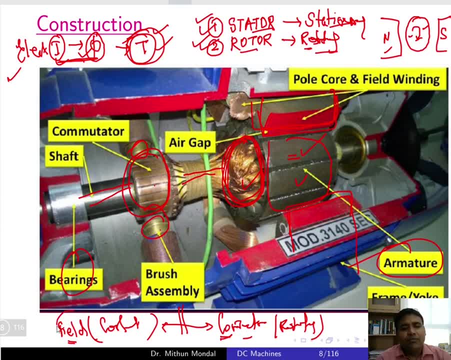 part. So in DC machine, as I said that the field will be constant, it will not be rotated. so which is the stationary part, The stator. so stator will have the field winding and the rotating part. so rotating part is basically the conductor. so the rotor will have the rotating part. so here your 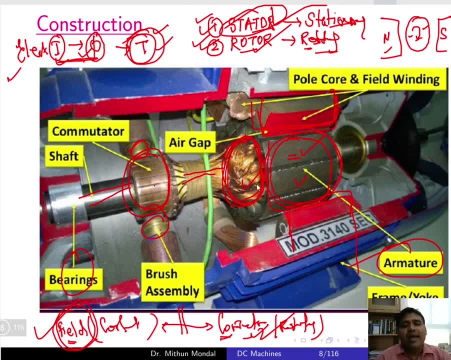 armature is basically the rotor, okay, and the conductor which is placed in the armature is connected with the commutator through the brushes and commutator is connected with the shaft with the help of a bearing. and the whole part, whole part, is present inside a frame. 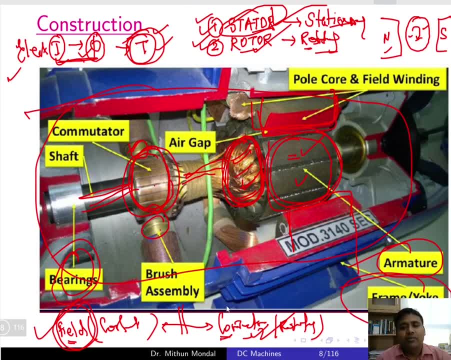 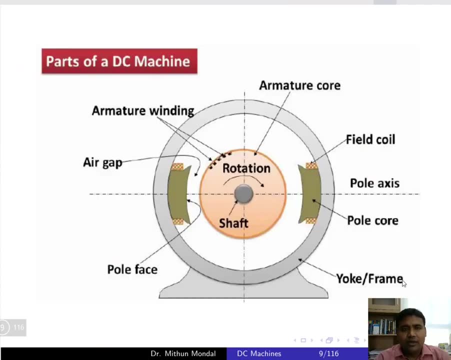 or a yoke to protect and the delicate machine. So the frame or yoke is to protect the entire machine. So this entire part is totally covered with the help of a frame or yoke. So this is the basic construction of a DC machine. now, if I draw it from a figure point. 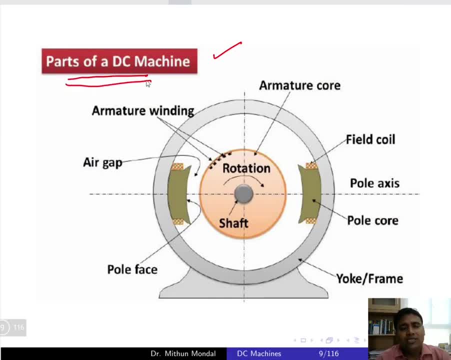 of view and we like to see the parts of a DC machine. so what are the parts of a DC machine? So let us start with that. so here, this is your rotor, This is your rotor And this is your stator. okay, this is your stator. 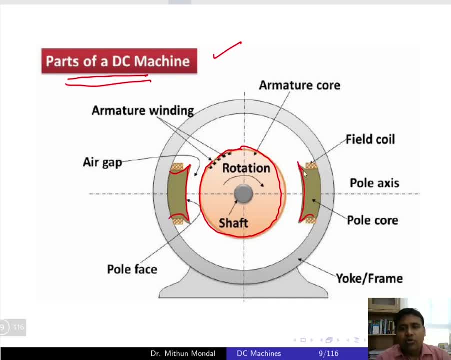 So stator is basically the stationary part and rotor is basically the rotating part. So this stator will be including the field coils, So the field coils here. field coils are present in the poles of the permanent magnet, So the field coil is responsible for the production of the flux. 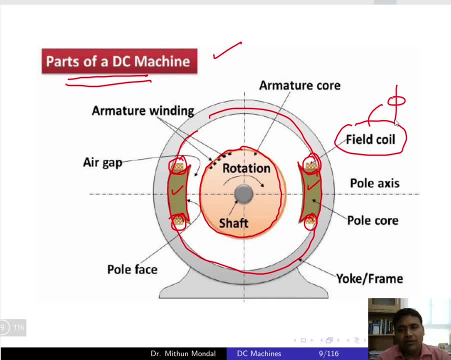 Field coil is responsible for the production of the flux. and these are basically the two poles, north and south, And this is your pole axis which is passing through the centre. This is your pole axis which is passing through the centre. Now, if you see, there is an air gap between the poles and the stator. 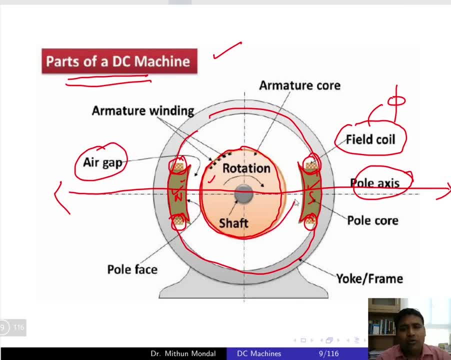 So there is an air gap between the poles and the stator, the rotating member of the machine. so there is a air gap. so this is your air gap which is present between the poles of the magnet and the rotating part, now the rotor, which is rotating. we will be using the term rotor or armature. 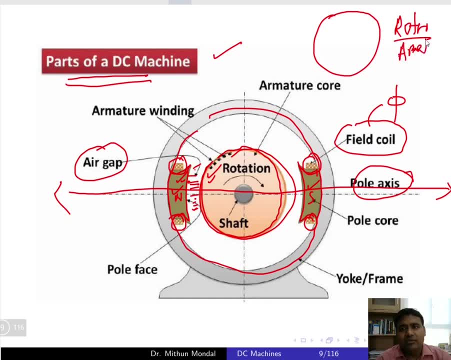 anything. both meanings the same here in case of your DC machine. so rotor and the armature is having the same term in case of the DC machine because the armature is the one which is rotating and armature will have the slot which will be carrying the armature winding. so in the slot the armature winding will. 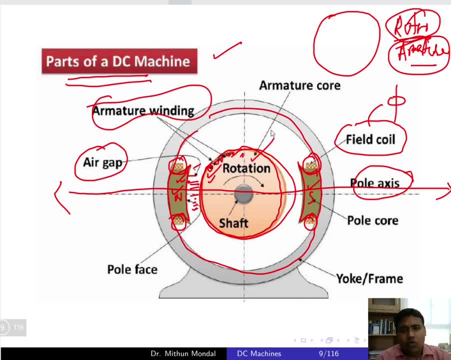 be present and this is the armature core. so the poles will have symmetry told to and below these vertical lines. so basically, this is a some face. so poles will be like this. so this is known as pole face. so pole face is this one, okay, and the entire machine is present in the yoke or the frame. so this we have seen as the physical. 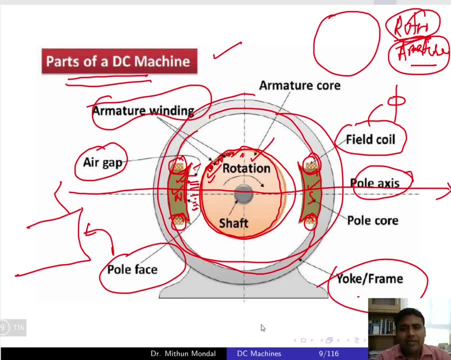 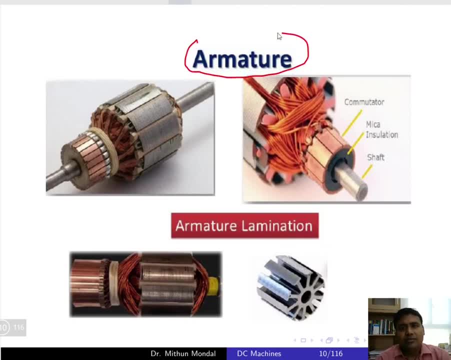 machine also and from the diagrammatic representation also. so let us concentrate now on armature. so let us concentrate on armature first. so here you have seen that this is your commutator, so this part is basically the commutator that you have and this is your shaft, which is rotating. okay, and between the commutator and shaft there is one. 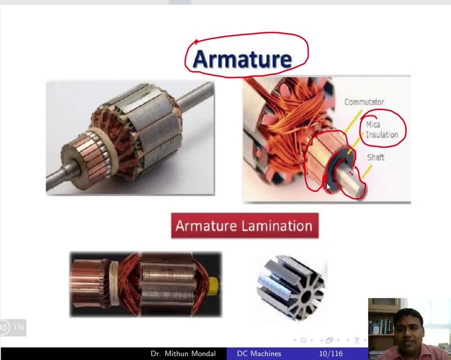 mica insulation. between the commutator and shaft there is a mica insulation and here you have the conductor. So these are the conductor which is present in the armature slot. So this is your armature, this is your armature and the conductors are owned and present in the slots of the armature. 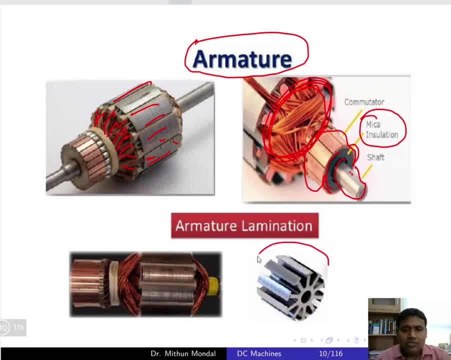 Moreover, the armature, if you see, armature is not a solid one, rather it is a laminated one, Like we have discussed in transformer core as well in magnetic circuit- we see that while laminations are required- you remember that we have talked about eddy currents, So eddy current. 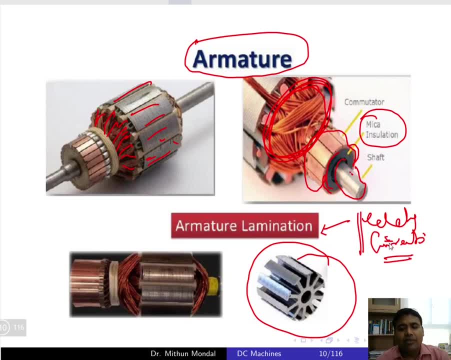 has to be minimized, and this eddy current can be minimized only when the resistance is more, and this can be done when we decrease the area. So if we decrease the area, which means that we have to laminate the core of the armature. So if you see this armature that is being 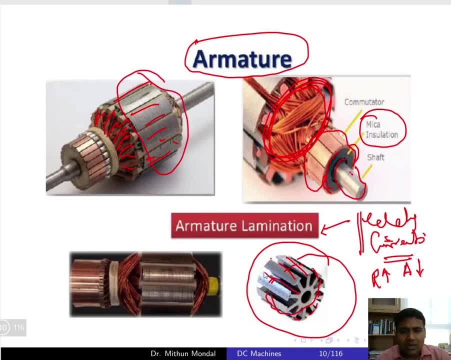 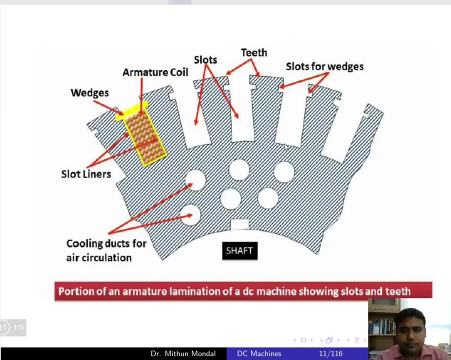 laminated and in the here in the core, you will be having all this armature winding. So all the armature winding will be present inside and then it will be coming out and connected with the help of a commutator. Okay, So if you see the portion of armature lamination of a DC machine which is showing 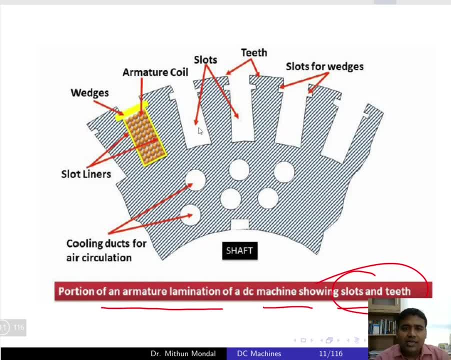 the slot and the teeth. So you can see, here you have the slots. So these are the slots which is present in the armature. Okay, And in these slots you are having the armature winding. So these are armature coils. 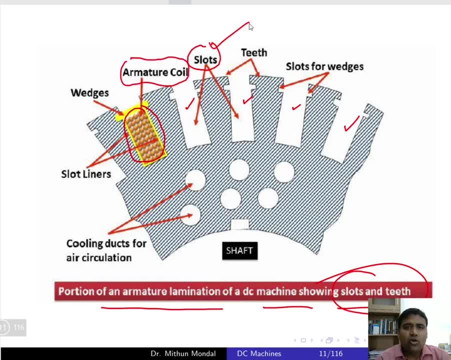 So armature coils are present in the slots of the armature, which is in the form of a wedge And there are two slot liners and it is in the form of a teeth. So you can see that this is in the form of a teeth. So this is connected in the form of a teeth And you have some slot for 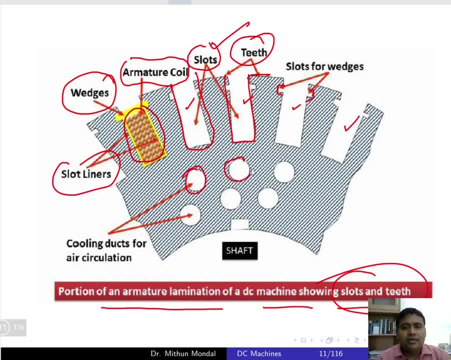 these wedges. These are present in the armature to cool ducts for air circulation, So that there should be circulation of the air, because you know that this conductor will be responsible for production of the heat because of I square R loss. So I square R loss will result in the 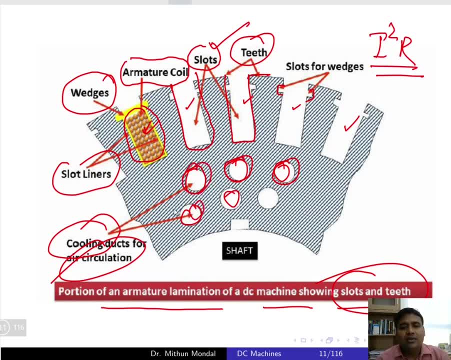 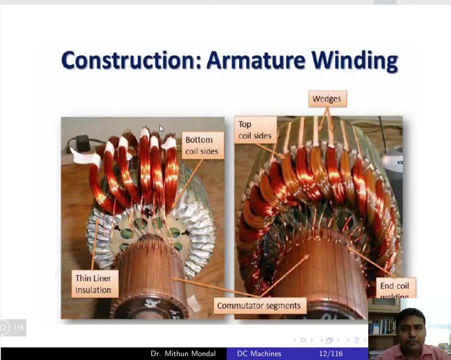 production of the heat. So you should have some cooling duct here for the air circulation. So in this way the conductors are present In the armature Now the armature winding construction. if you look, then you will be. 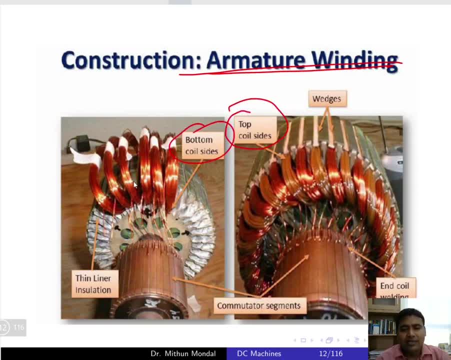 having some top coil side and bottom coil side, So that will be present And this is very complex in case of the DC machine. So because of that the cost of the DC machine is quite high. So as I said in the discussion, the limitation, the cost is high in the DC machine because of 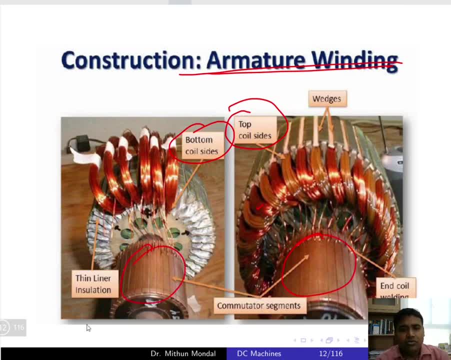 this armature winding and the commutator. So because of this commutator and the armature winding the cost is quite high And you will be having the mica insulation between the commutator and the shaft, So that you have- And here you. 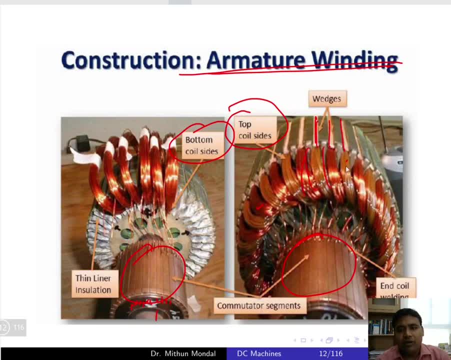 have the wedges through which the windings will be coming, So these windings will carry the current and it will rotate. So it is rotating in what? So it will rotating in the field. So, as I said, the field will be there, north pole and south pole. 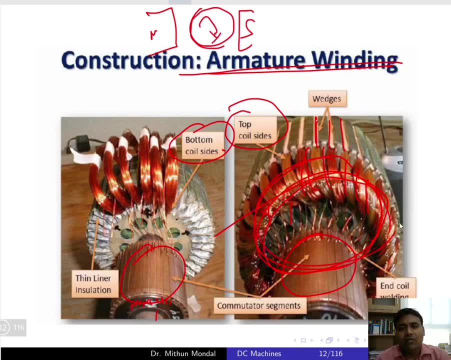 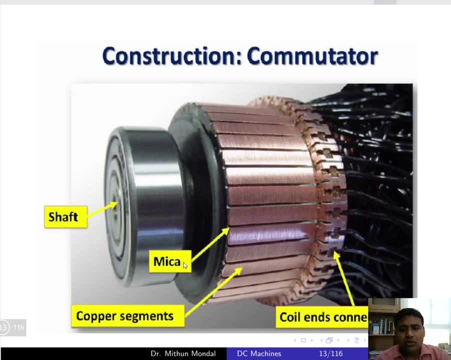 So you will be having an electromagnet which is rotating And this electromagnet is basically this armature windings. Now, if you closely look into the commutator and the shaft, as well as the insulation, So you can see that the coils which is coming. it is basically 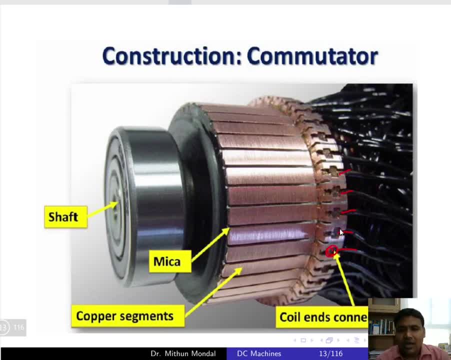 connecting in some segment, So these are known as commutator segments. These are known as commutator segments, So coils are being connected in the commutator segments And here you are having some mica insulation. Mica insulation is there And these 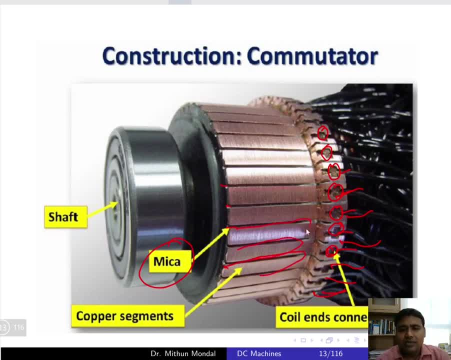 commutators are having the copper segments. So these are the copper segment And this is the shaft which is rotating. This is the shaft which is rotating Now when you are operating the machine as a generator and the mechanical energy through this shaft will be converted to electrical energy, And when you are using as a motor, this shaft will be rotating and giving the torque outside. So that is the connection. So here one important point is the commutator segment that is present in the commutator. 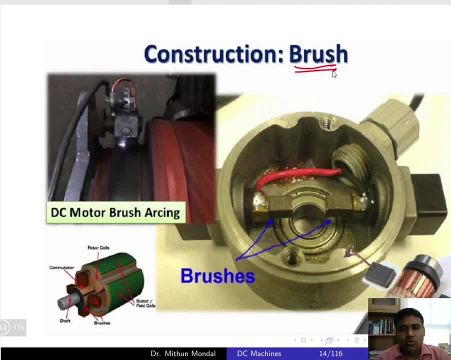 Now the next thing that we will discuss: the brush. So where is the brush? So you can see that there will be two brush. This is one brush, This is the other brush. So the brush is made up of carbon, So the brush is made up of CARBON. So two brushes are there, which is? 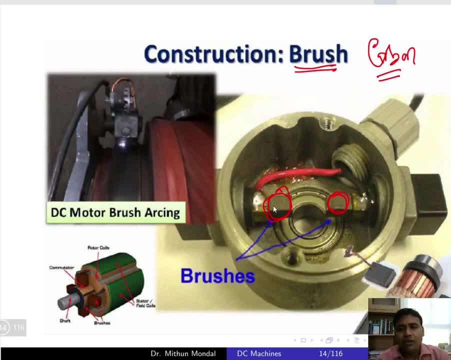 connecting and keeping fixing on the commutator. So since it is continuously rotating, this brush which is attached to the commutator will get produced a spark. So there will be the production of the spark and the brushes will be wear and tear shape. It is not permanent. 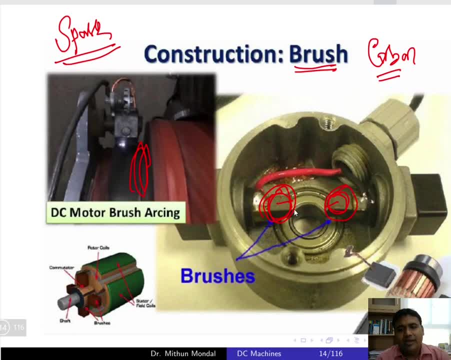 will be there in the brushes, so there will be wear and tear of the brushes. so this brushes being shown here is a carbon brush which is sticking with the commutator, which will be like having wear and tear and there will be a spark produce in the brushes, so there will be arcing. so there. 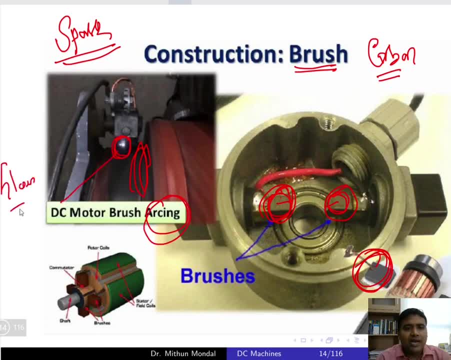 will be some arc, so glow will be there. because of this arcing you can easily see with your open eye, so there will be glow. so because of this commutator and the brush and the armature connection, the cost is increasing and the dc machine is becoming quite complex. 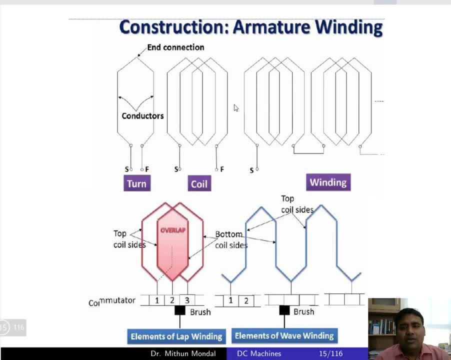 now we will introduce some term for the armature winding. so we have seen the armature winding will be present. so one term is known as a term, other term is known as a coil and the third term we are using as winding. so why is that? 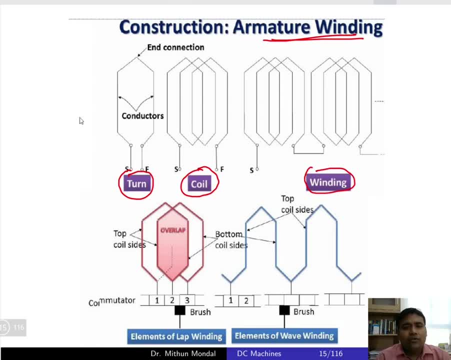 So what is a term? So term consist of two conductors, so other term is conductor, so conductor number one, conductor number two, which is connected in the end. so both conductor are connected and the other part of the conductor. we are taking it out so you understood that one term is made up of two conductor, so 2. 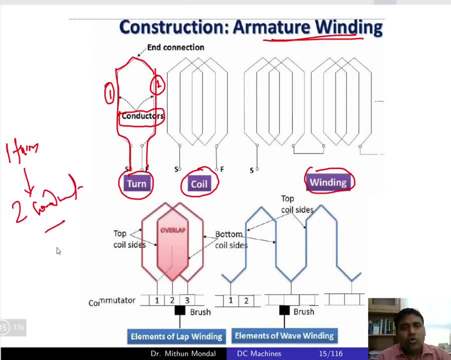 conductor will make 1. Now, so many turns. so many turns will make one coil. so many turns will make one coil. so many coils will be connected to form a winding, and this is the armature winding. So we have started our discussion from conductor. 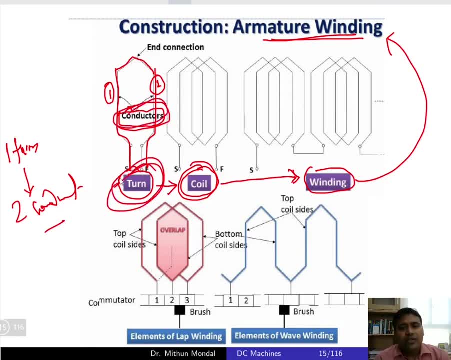 So two conductor will make one turn, so many turns will be connected to form a coil and so many coils will be connected to form a winding. and this is what the armature winding is, there inside the armature slot. Now let us see the commutator segment. 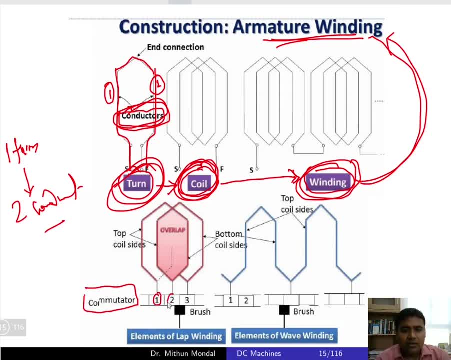 So here you can see that commutator segment is there: 1,, 2,, 3 and so on. commutator segment, So the ends of the coil. if you see, the end of the coil is coming and connecting with the segment of the coil. 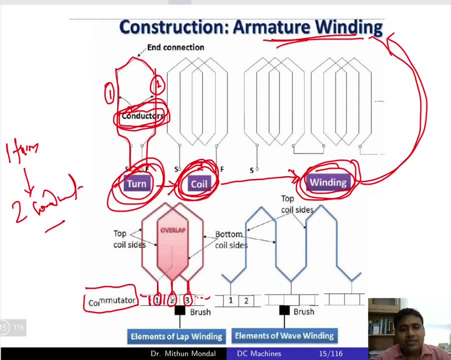 This is the commutator. So these commutator segments are the one which is holding the armature conductor and these, if you see the segment, if you see the segment, it is continuously rotating. this armature is continuously rotating and the segment is present in the commutator and the brass is. 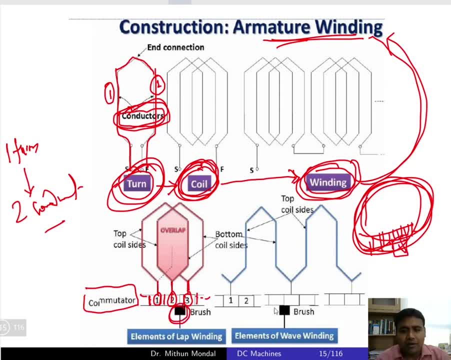 associate is tapping on the commutator, which is carbon. So the brass is tapping on the commutator segment And the supply, either input or output, is taking from the brass. So if you have this is your armature, ok, So we write it to be a machine M. this is your armature and the two brasses we represent. 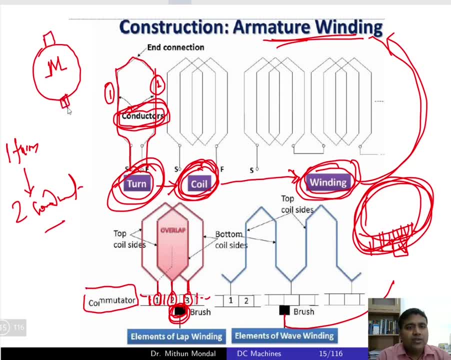 which are sticking to the commutator. So these are the two brasses, ok, and either the input or the output will be taken from the two brass. So in case of your generator, the output energy will flow in this way in case of your motor. 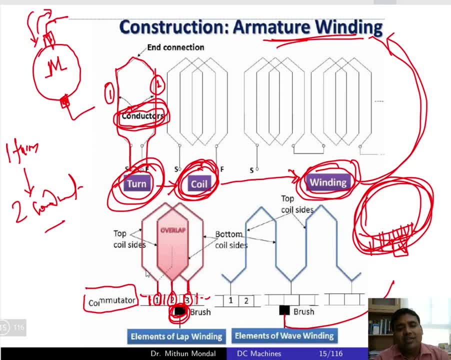 the input energy will flow in this way, So the electrical energy, either taking or giving, will be through the help of a brass, and that will be given to the commutator segment, and here the armature windings are there. ok, So this is about the commutator segment. 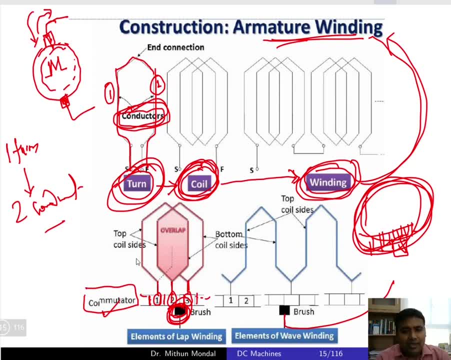 Now let us discuss the coil side. Ok, So if you see, the coil can be connected in two different fashion in armature. There are two different fashion by which the coil can be connected in the armature, So these are basically the lap winding and other is wave winding. 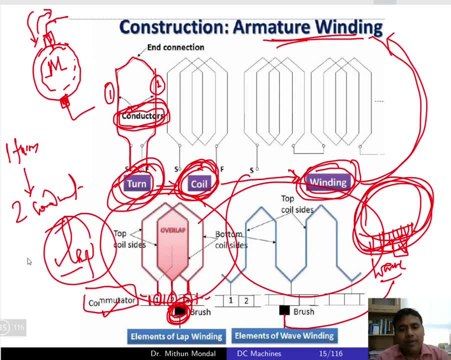 Lap means: if something is moving back, that is lap, if something is moving ahead, that is wave. So if you see a wave, it is always moving ahead. it is not moving back, right. So that is a wave. if something is moving back, that is lap. 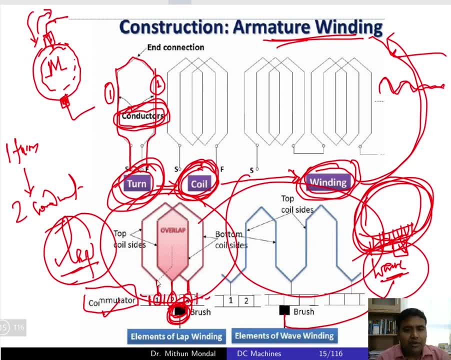 So if a coil has started from the commutator segment one, then we can move and go ahead with this side here, this way, and then from here we will move back and this way. So this is known as the lap winding, Because it is moving back. 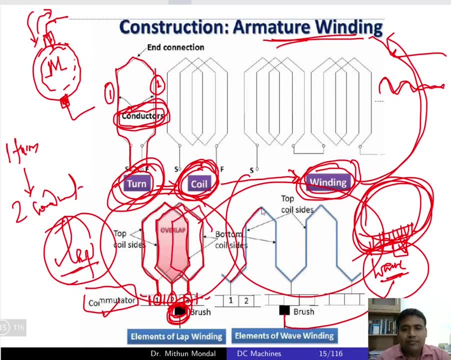 If you see the wave winding, so it will move front. So something which is progressive and something which is retrogressive. So if there is a progressive, then it is a wave winding, if it is retrogressive, then it is a lap winding. Ok, 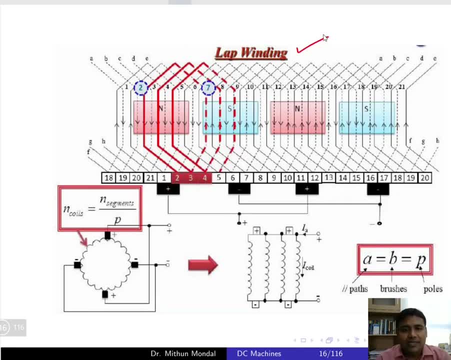 So, if you see the lap winding in more detail, so let us see the commutator segment. So here you can see the brushes are there. So this black one is basically the brushes. Ok, Ok, Ok, Ok, Which is attached with the commutator. and these are basically the commutator segment. 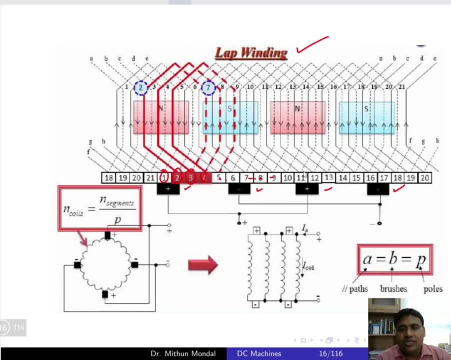 1,, 2,, 3,, 4,, 5,, 6 and so on. So these are the commutator segment, and from the commutator segment we are basically taking out the armature conductor which is connected in the form of a lap or the wave winding. 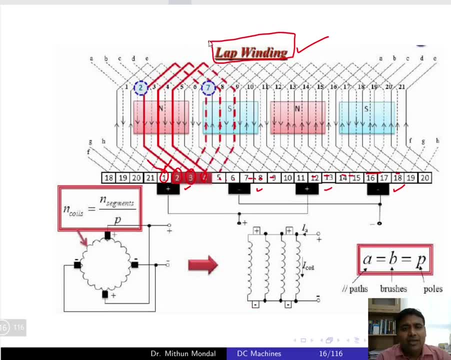 So the first winding, we are considering the lap winding. So if you see the winding number 1, and is this So here? what we see, that if you consider this- coil number 2 and coil number 7, what you see that the coil number 7, if you see that it is coming at 3 and coil number 2 is starting. 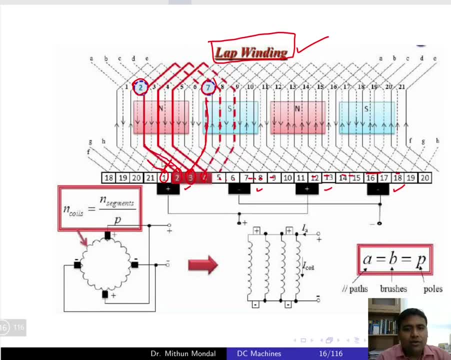 at segment number 2.. So from the segment number 2 the coil side has started and then it has moved and then finished at coil number 7, which is at commutator number, segment 7. So all the commutator will be divided so that any coil side which has started will flow. 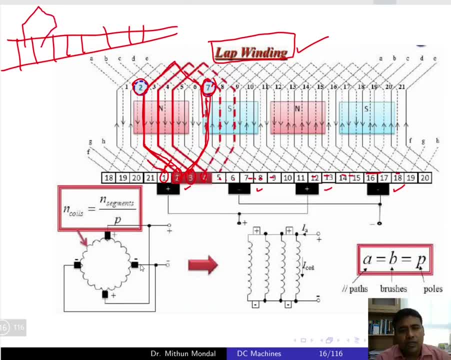 and then it will stop in other commutator segment. So the number of coils will be number of segments divided by the number of poles. that is which we have, And through these brushes, energy will be tapped. so this brushes, energy will be tapped. and one point that you have to remember here in lap winding is this: one number of paths number. 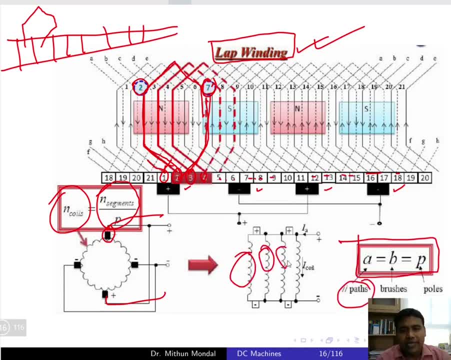 of parallel path. so this is parallel path 1, parallel path 2. like this, Number of parallel path is equal to number of brushes, is equal to number of poles. So whatever the number of poles, you have the same number of brushes you will be having. 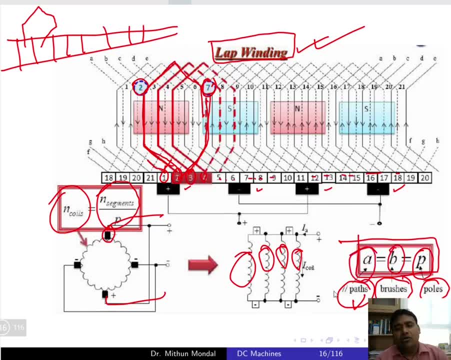 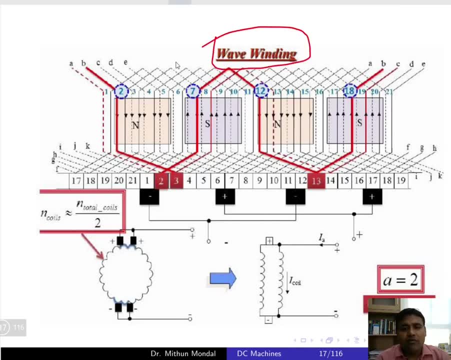 And same number of parallel path will be having for the current distribution. So this is lap winding, If you see the wave winding. if you see the wave winding you will be having. the number of parallel path is constant as 2.. So number of parallel path a is equal to 2, always. 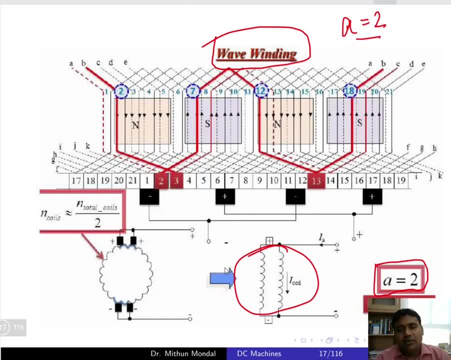 So there will be 2 parallel path in the wave winding. there will be 2 parallel path in the wave winding And the number of coils will be equal to total coils divided by 2.. So in the previous case we were dividing with number of poles. here will divide with the. 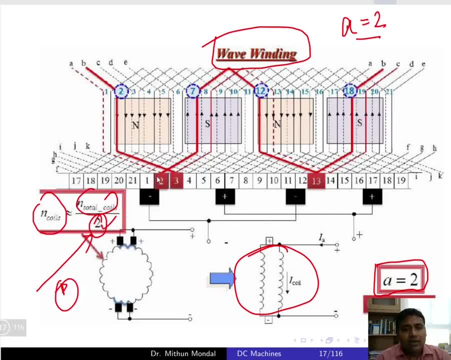 number of 2.. So here in the commutator segment, if you see, so these coils, which is started from 3, if you see here, so it is moving here and ending with 2.. So it is just progressing. it is just progressing, you see, it is not coming back.